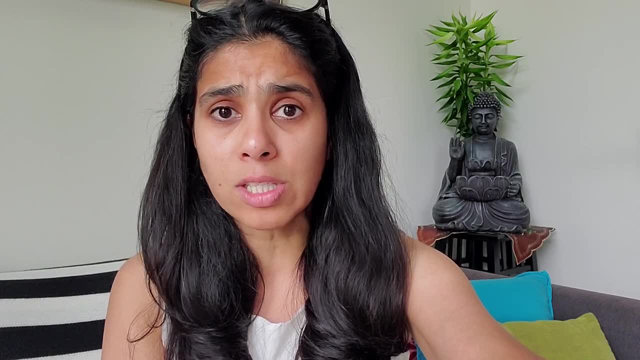 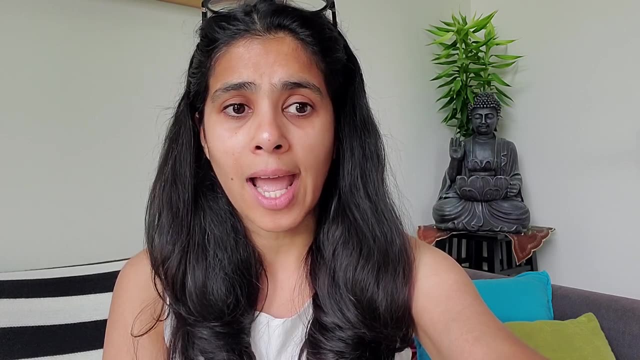 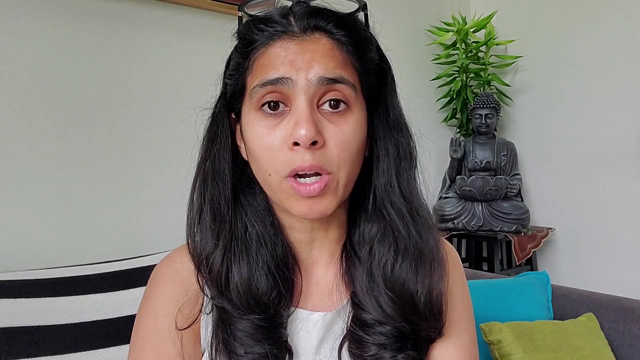 learning style, or you could say visual spartial intelligence, which refers to person's ability to perceive, analyze and understand visual information, and basically they can picture the concept in the brain and they will be able to solve it. So that's what we are going to be focusing on today for kids. 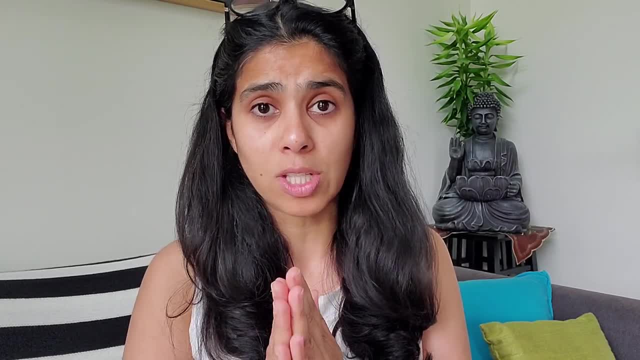 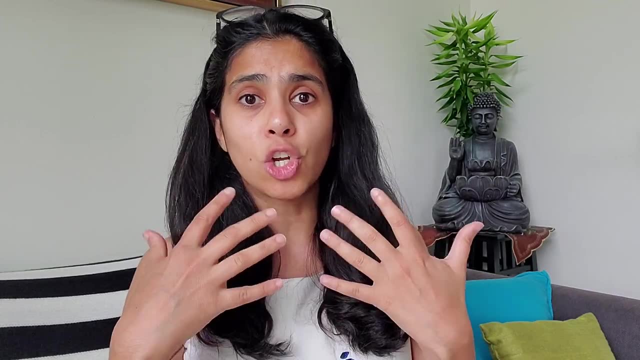 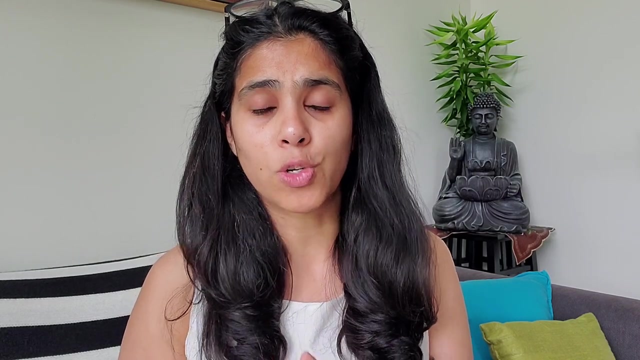 but trust me, for the brain and for the visual intelligence they are very intrigued. There are so many things that are going on in that activity that you might see your child engaged for a good 40-45 minutes with just one activity. Alright, and definitely, as I always say, you can when you're. 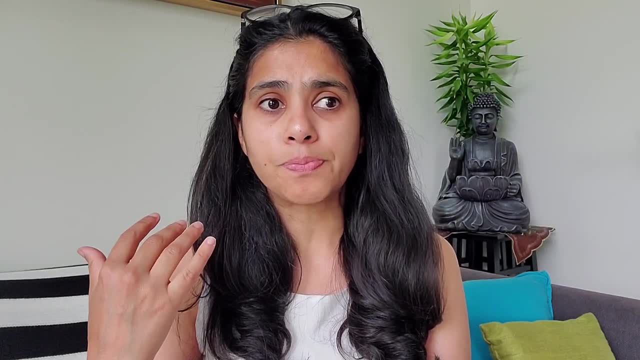 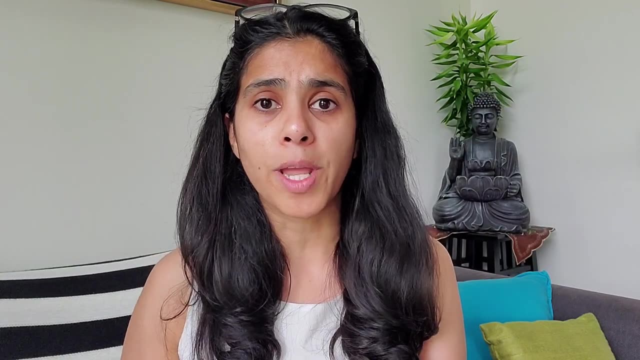 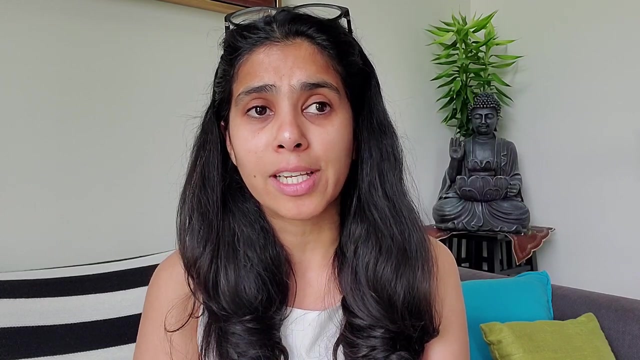 recreating the activity. you can always make sure that you're adapting to your child's interest in that activity and I am making that's the perfect way. you could always take a level up or you can take a level down. So before I get going I just wanted to make sure and tell you guys that the 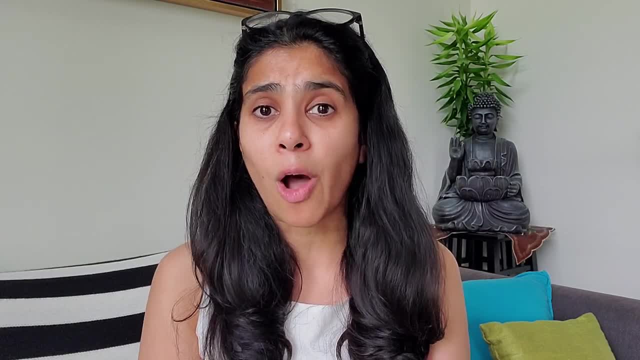 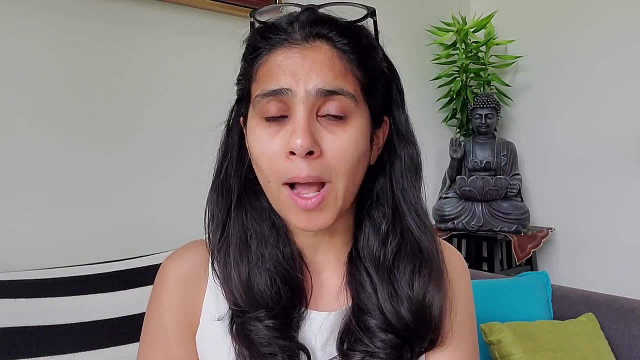 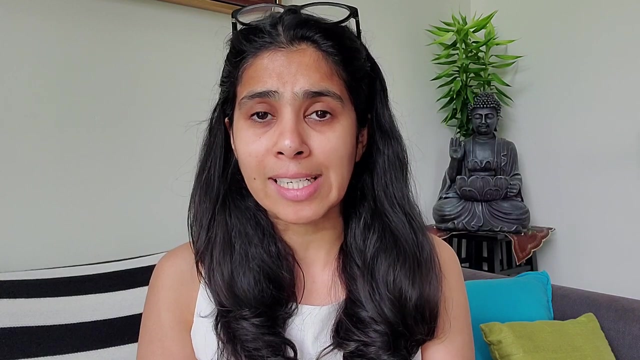 giveaway which was going on. I have got a great response, however, that I have got some information from YouTube which says that the people who had participated- alright, and the subscribers that came in, they have left. So I am just trying to get the details and I think they're. 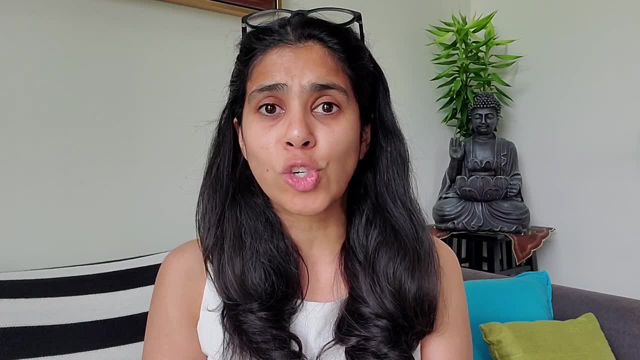 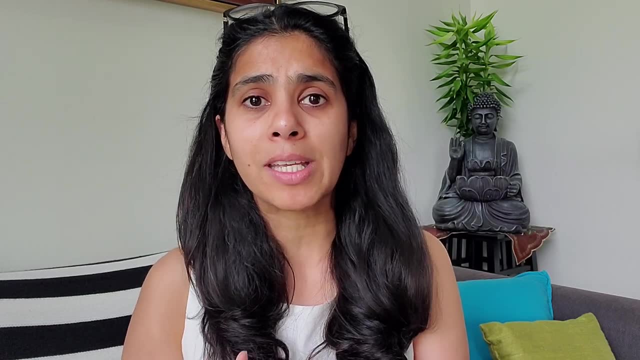 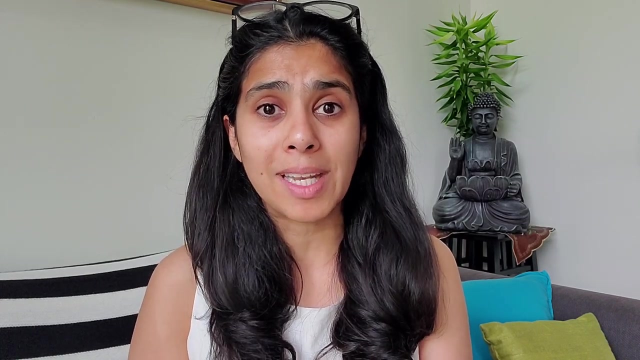 going to get the details and I might need to void that giveaway because it's really getting a lot of trouble for me and I'm getting a lot of emails from from YouTube itself because of subscribers coming in and going and not following the rules. So I think I'm going to do a detailed video on. 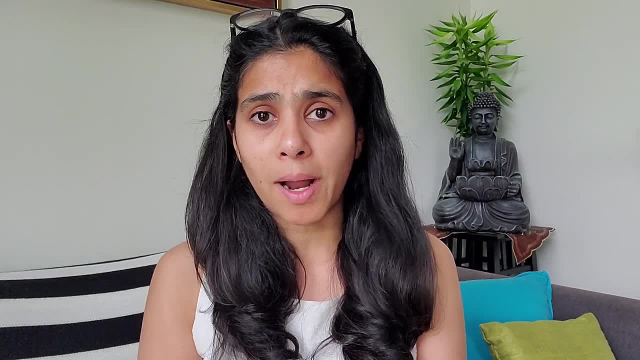 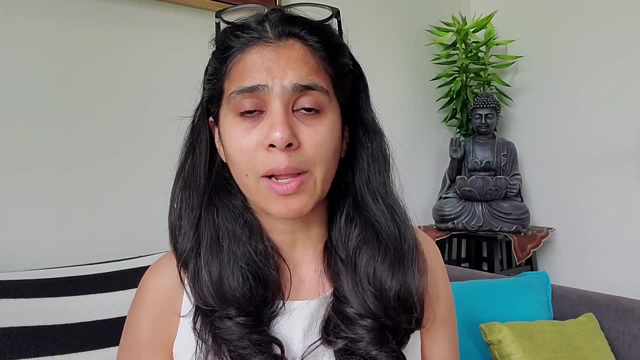 this, maybe next week. I'm still gathering data and working on it, but just wanted to give a heads up that if you've already participated and if you see that the people who came in through you if they have, if they have done it, then I would just say thank you so much for watching and I will see you. 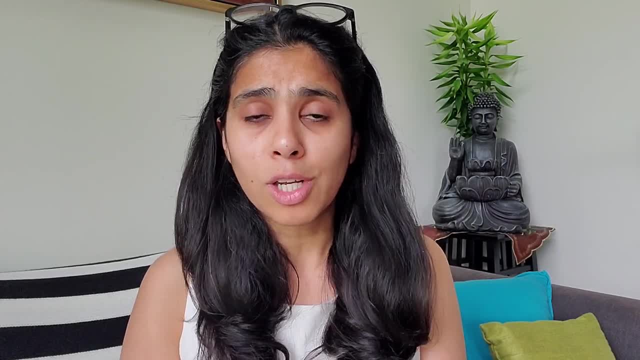 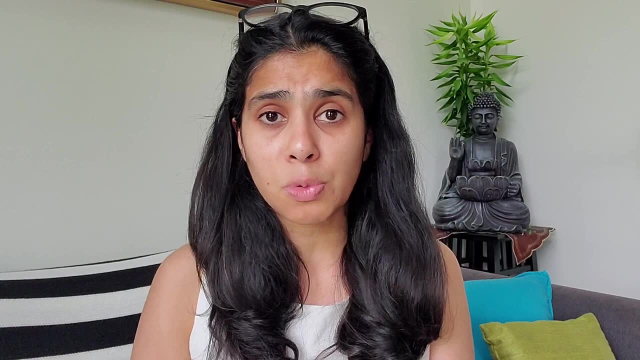 in the next video: Bye, Please. that's not really very, very cool to do it to to get $150, and there are a lot of spammers, definitely. so I'm just trying to figure this one out. Okay so, but just one more thing, guys, if you. 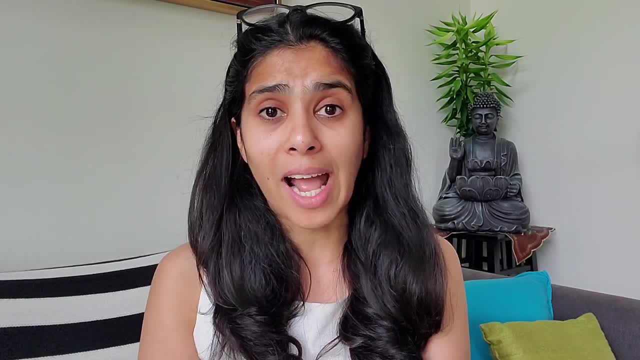 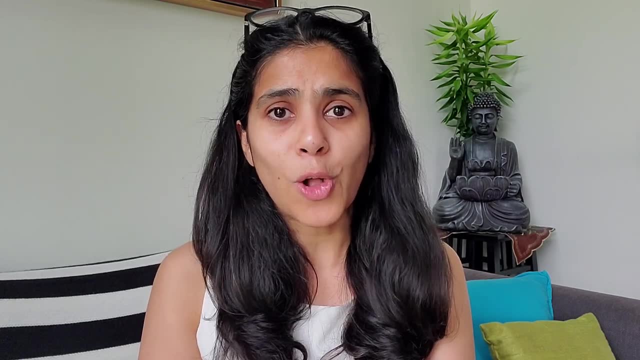 need the printable for this one, the one that I have made for Vivan. I would want you to please leave a comment. it's on request basis and I can share the file with you. Alright, so leave your comment in the comment section below, in case, if you need this file, I will be able to share it with. 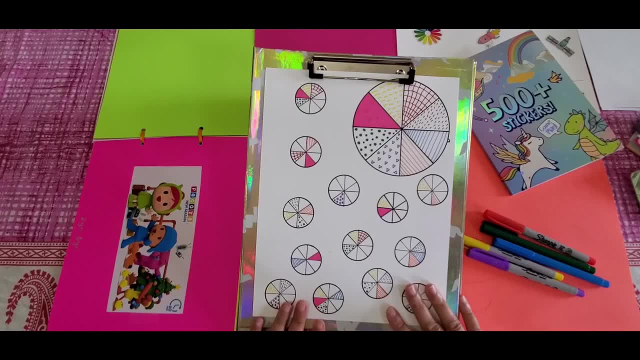 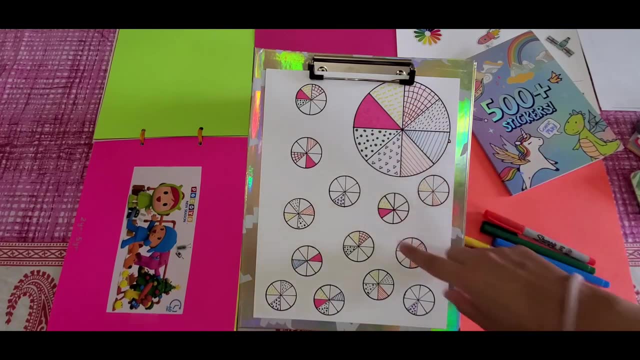 you Okay. so let's get to the first activity, and this is like a wheel that I've created with using a circle, and if you would see, this is a big one, and then you have these smaller ones that I've created here. so now, because the video is all about visual spatial intelligence, so there are so many. 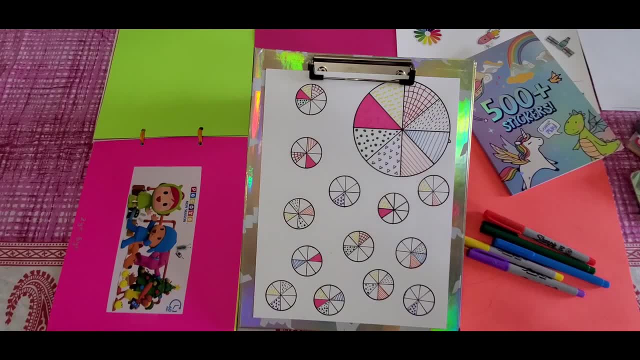 things that are going around here. so there are lines, there is a dots, there are triangles, there are, there is this grid that's going on. so every circle and one, two, three, four, five, six, seven, eight. so there are eight segments and then you have to create a circle, and then you have to create a. 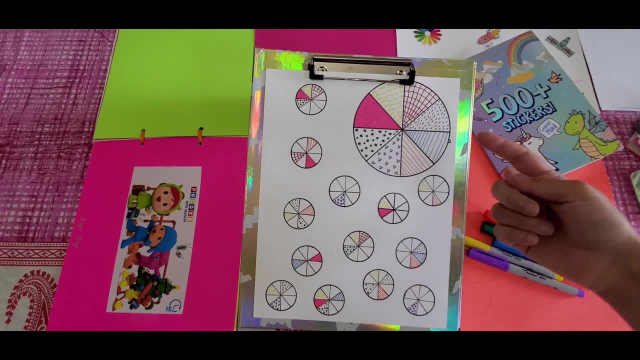 segment, and all eight segments have a different design or a pattern. all right, so what the child needs to do is here. then, when you see all of these right, they need to complete the missing ones, and trust me that I have not made it very, very simple, because I have made sure that they are turned, or? 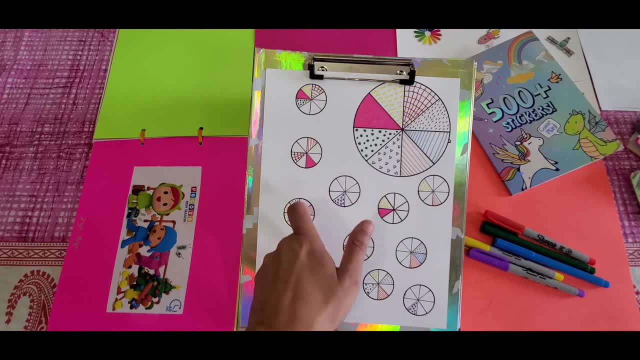 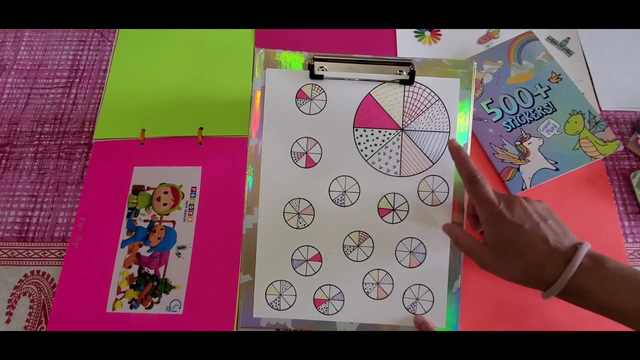 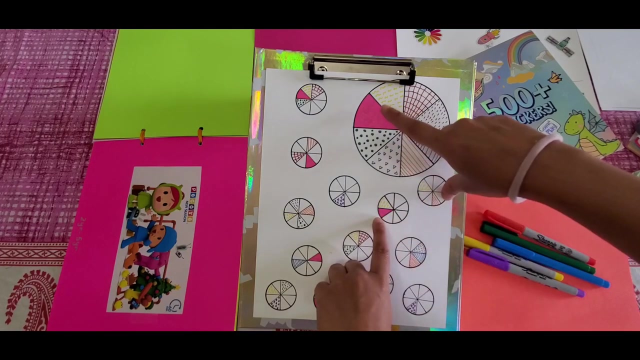 twisted somewhere, like just the way a wheel rotates right, so it is rotating in many, many different directions, so that, like, okay, let's take an example, like you, these triangles here and that triangle is right here. okay, so that's a similar spot and that's the same spot. however, the same thing now. um, you have this pink right here, but, however, this pink is. 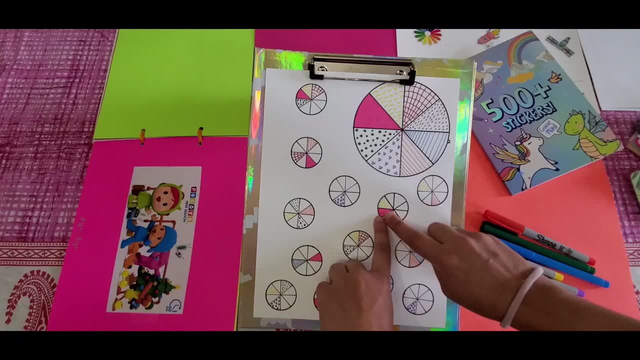 right here, right. so it was already moved and it is on this direction now. so what the child has to do, he needs to figure out the rest of them, and it's the same thing for almost each one of them that i have moved the shape like. so the green is actually here and i have moved the green right at 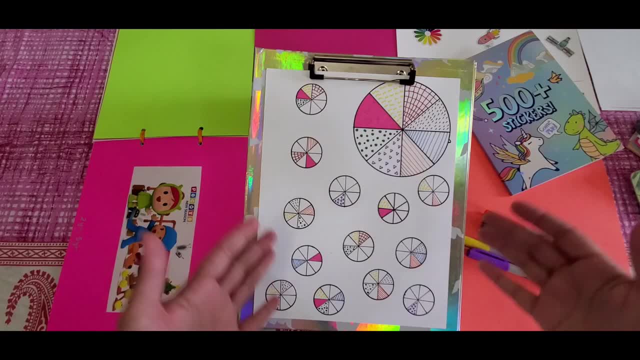 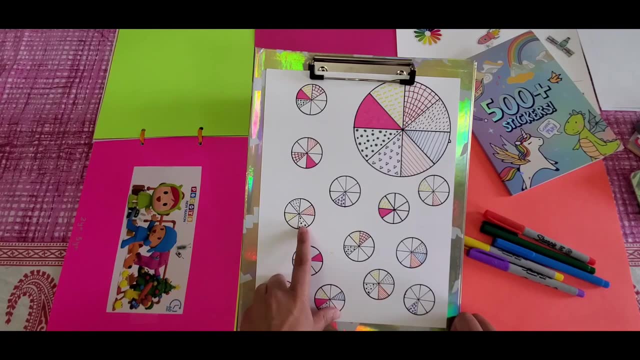 the bottom here. so, uh, the child has to actually move and rotate every time he wants to do this activity and he needs to make sure that next to the green what comes, all right, so he needs to make that. so, of course, i have used my sharpies and my pens and vivan will be able to access them. 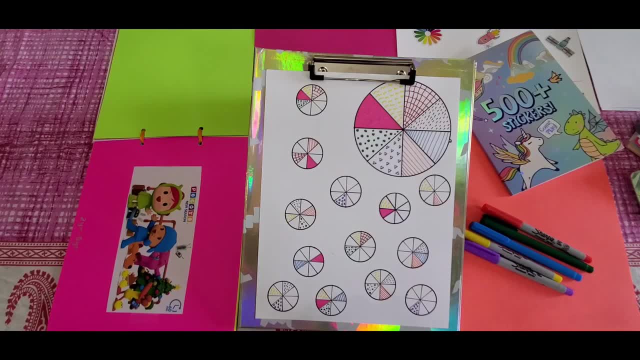 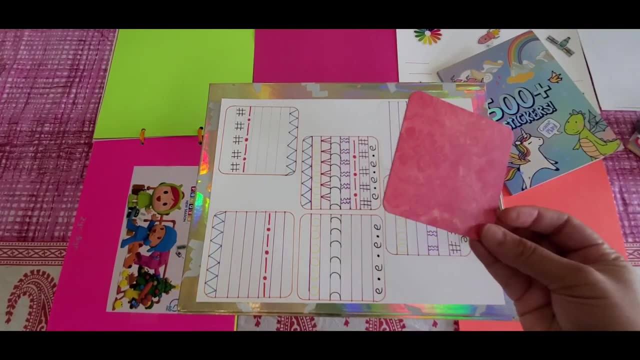 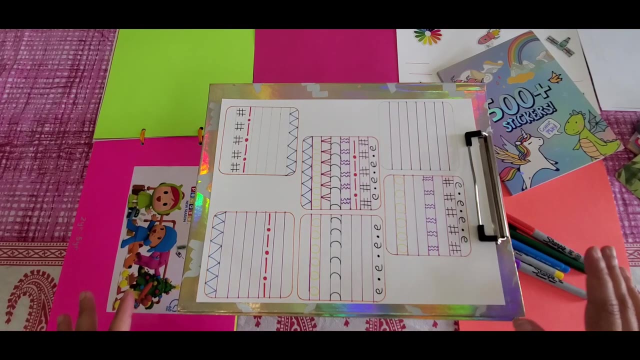 and would be able to recreate. let's move on to the next activity. all right, so in this activity, what i've done, i have, uh, i had used one of my square cards and made an outline for that and along with that, um, i have made some couple of lines here and some patterns. all right, 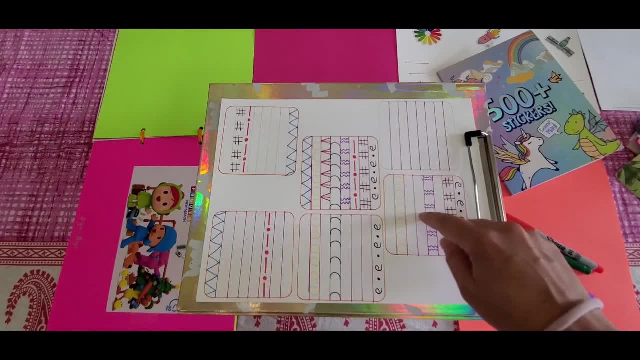 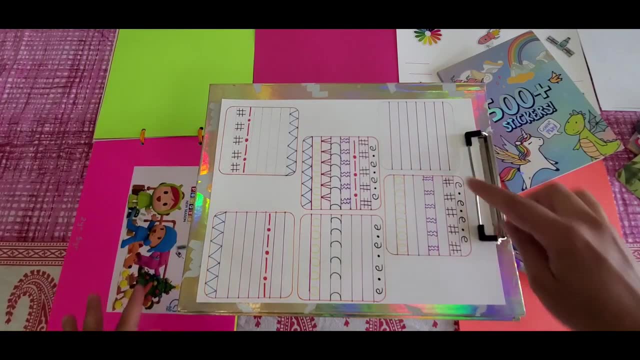 but here there are two things that needs to be done. so, because there are one, two, three, four. uh, one, two, three, four. there are six squares, all right, this one is incomplete and this one is incomplete. incomplete in sense of the border is not made here and the lines are not drawn here. 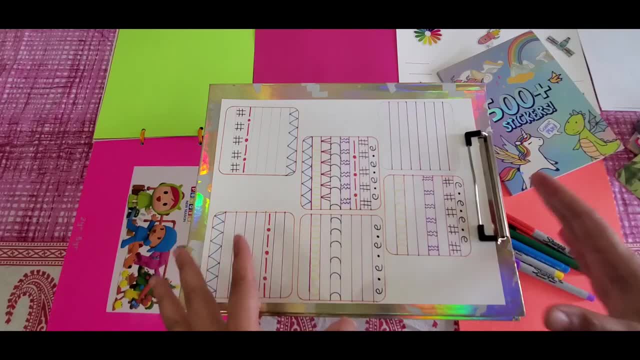 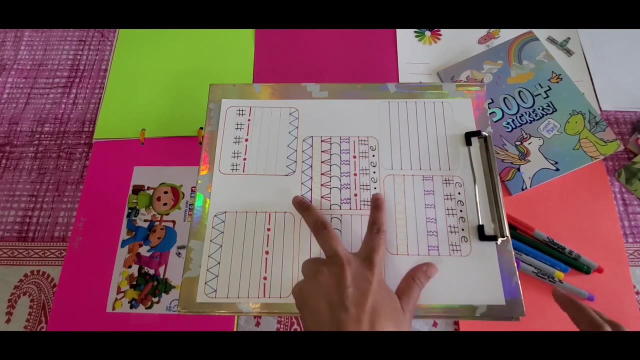 so that's something that he needs to make sure that he remembers that, because i'm going to be telling him- uh, i have not given an instruction here because i'm i prefer to give more listen here- and um, then he needs to finish this along with that i have. this is the main frame, okay, so 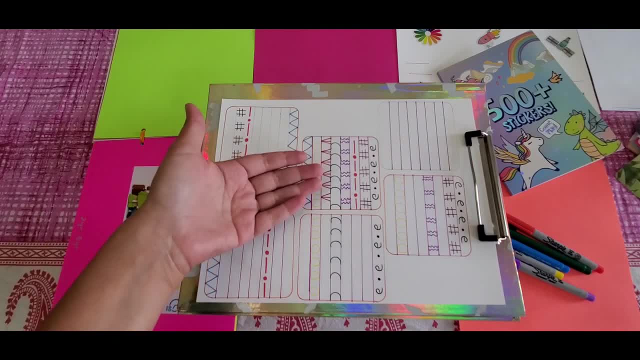 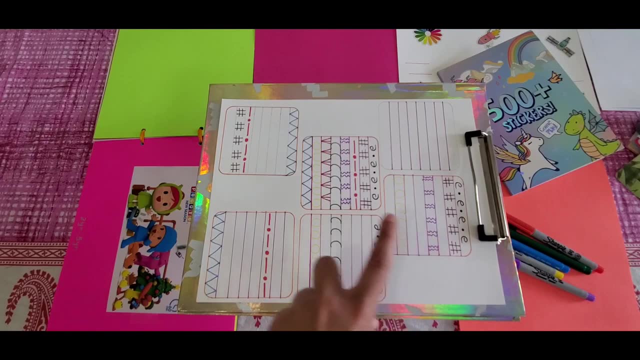 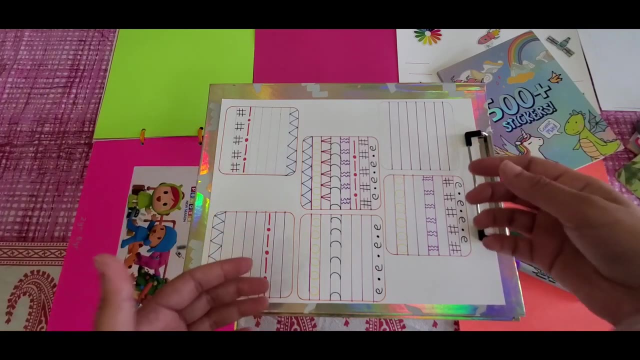 this is the main frame that i've created, and then he needs to complete that. what i've done, the same thing here. i have, uh, uh, made sure that i have turned this upside down here and along, uh, and this one too, so he needs to then keep flipping or keep rotating the page to figure it out how. 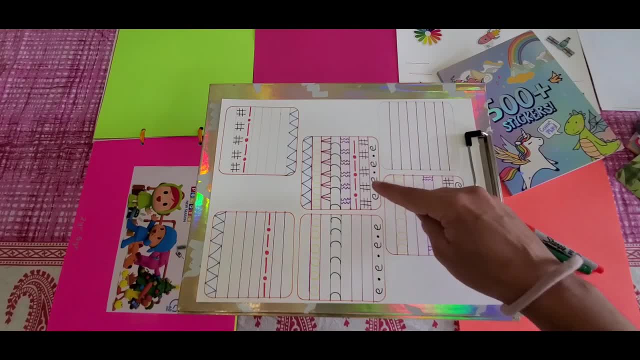 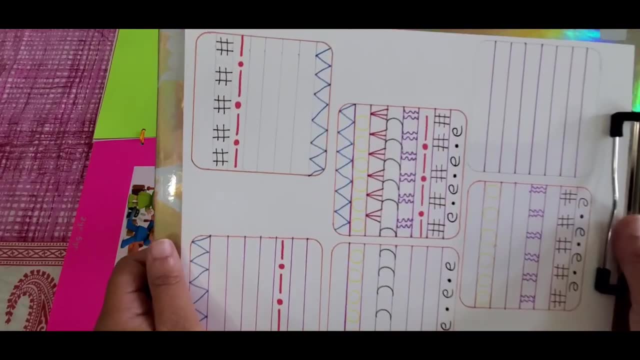 to complete these designs, and the designs in terms of the patterns are going to be the same. patterns have to come exactly where they belong. so it it might look very easy, but the way i've used the design, i'm going to show a closer look here. uh, if you would see, the circles are next to. 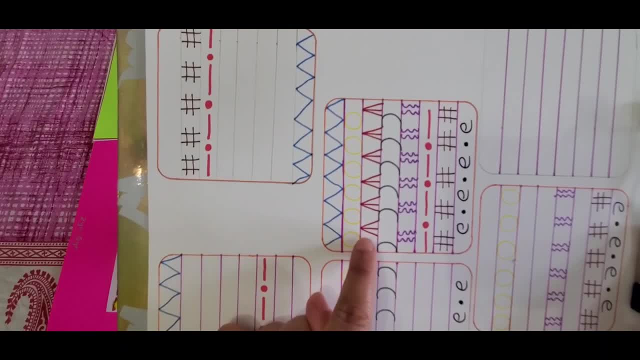 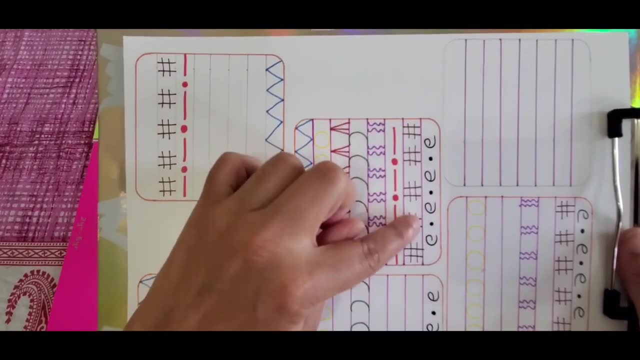 the points here, and the red is in between the two circles. so that's where our spotted intelligence and our observation uh is coming in. all right, and then we have four e's and we have three dots in between in the same way. so this is what the child needs to do. they need to make sure that they are. 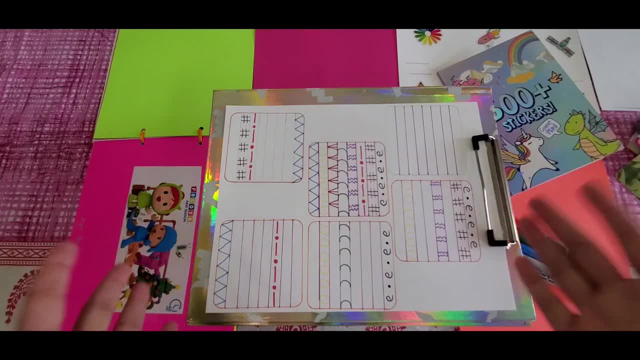 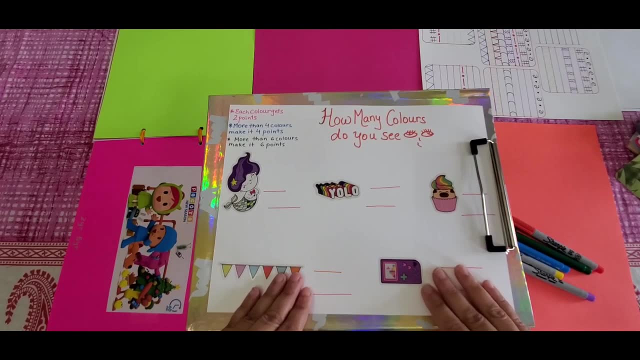 concentrating and, uh, they are able to recreate this. okay, so let's move on to our next activity now. all right, so this is more of a picture and colored observation and because it's for six plus- and vivan is almost seven and a half, he's going to be doing this. how have i made this so interesting and 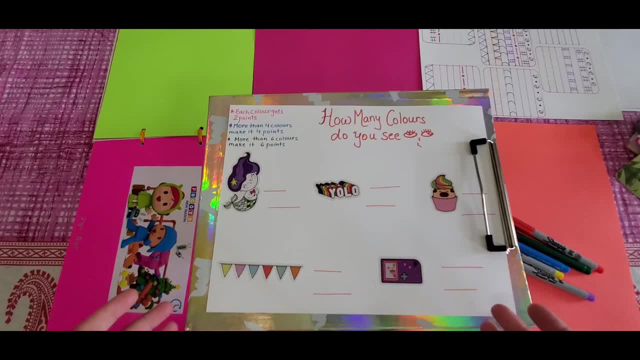 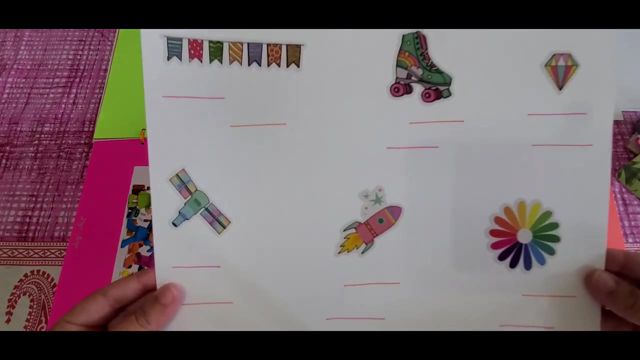 what is visual, uh, uh, how are they going to analyze and what are they going to observe here? so, if you see, it says: how many colors do you see? and i have used some very bright pictures like: uh, there are five or six゜, five pictures here. along with that, there are six pictures here and you would see they are extremely. 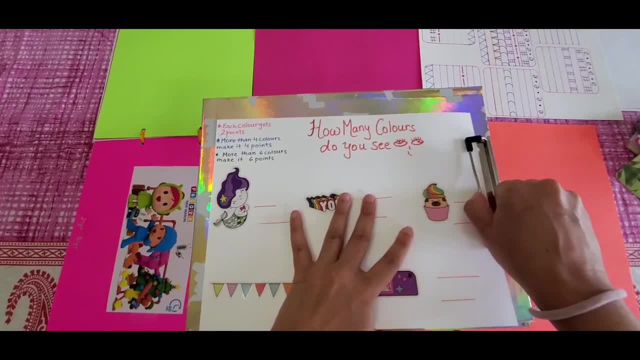 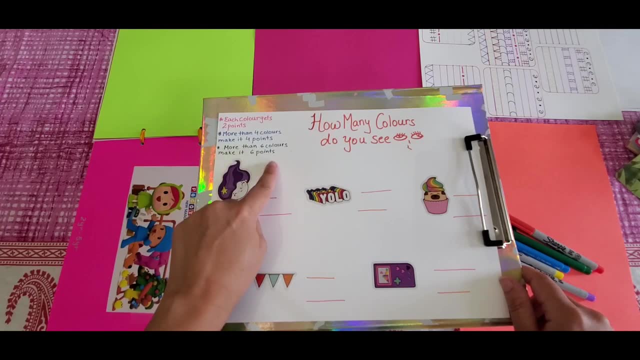 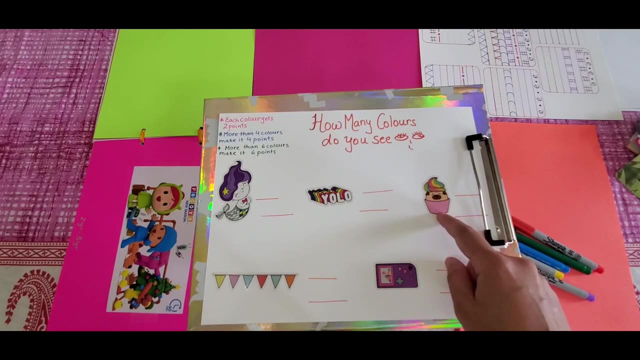 colorful right. so what i've done here is: i have given points, so each color gets two points. more than four colors make it four points, and more than six colors make it six points. so just imagine that, if he has taken this all right and he figures out, there are only four colors, so every color is four. 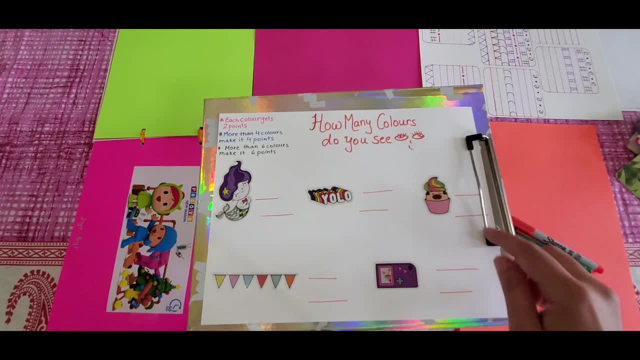 points and then he needs to add up and he needs to write it here. okay, so first he's going to write how many colors and then he needs to total up and add up the points. then if there are six colors here, so he needs to add that those he needs to write here six colors, and then he needs to add up, like: 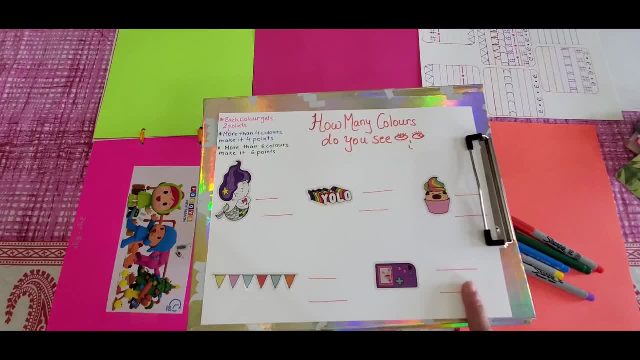 six into how many times the color is, and he needs to write it here. and if there are more colors like more than six, then the points are 12. okay, and you can keep it 10, 13, 14, whatever you want. i mean, that's how. 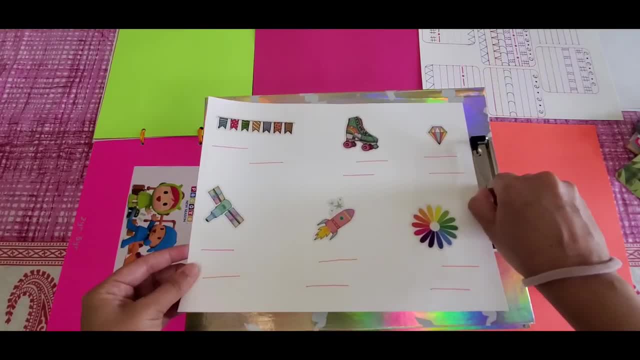 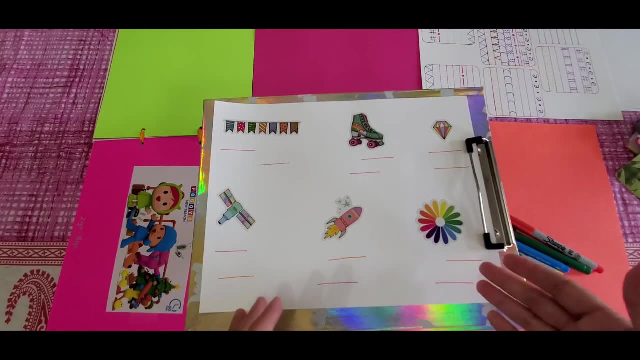 i thought i'm gonna build it. uh, same goes here. uh, you could see there are more than six colors here, definitely, and that's how? uh, like 12 or 13 could be a perfect way for this one or this one or this one. so it's a very, very 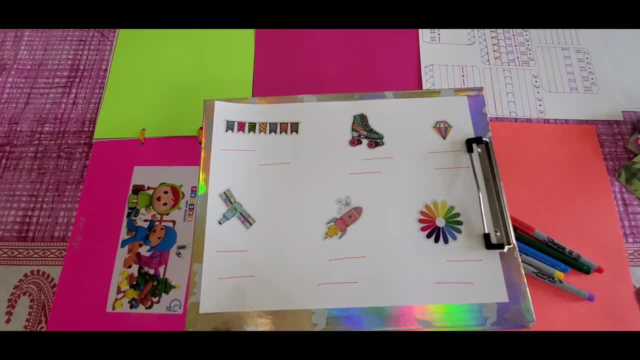 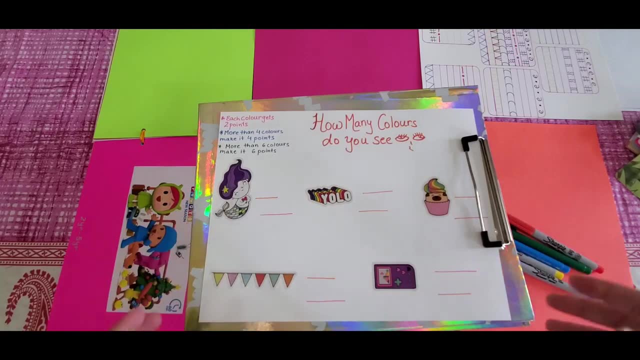 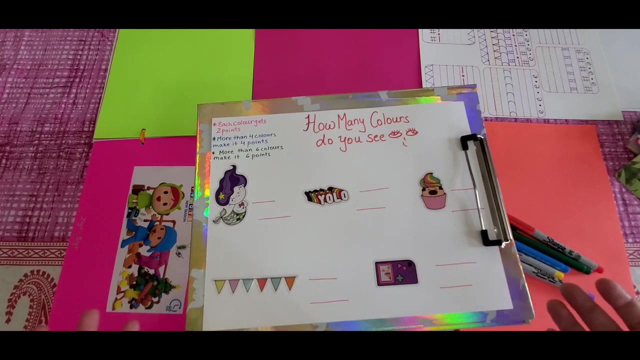 intriguing activity for a seven and a half year old, from six to eight. i think they'll be like really enjoying this activity if you uh make sure that you give a higher number so you can always give the number according to your child's age and uh um, in terms of addition or multiplication, whatever you want them to do and like this, this is a great. 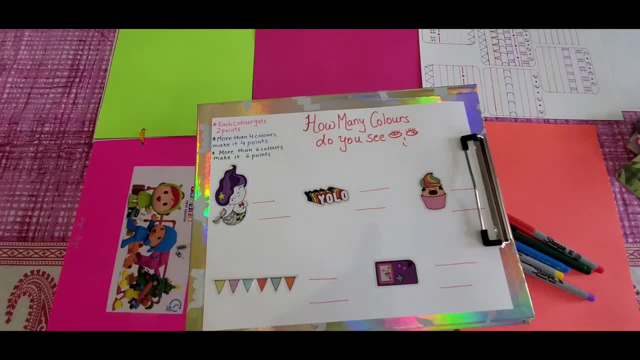 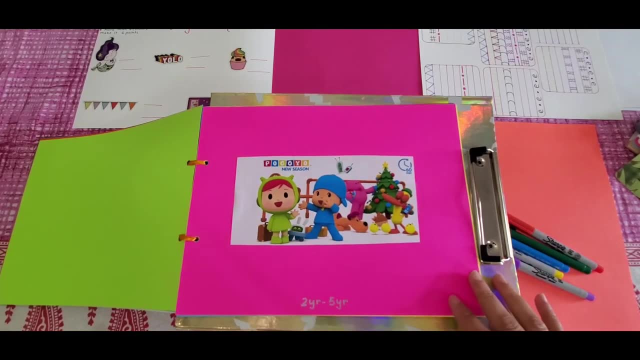 um, spartan intelligence, a visual spartan intelligence activity. let's move on to our last activity and let me show it to you. all right, so my last activity here: i have used vivant's baby book, where i had created the cartoons that we want watch, and how am i going to use this for visual spartan right? 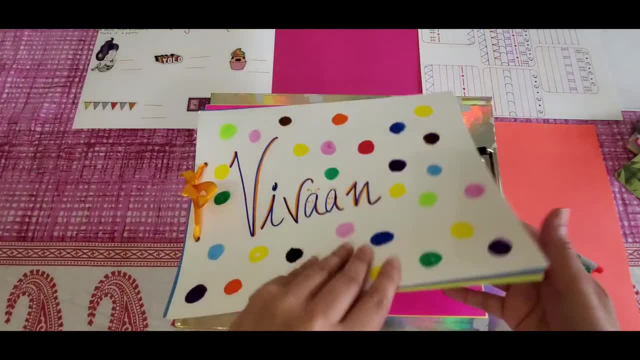 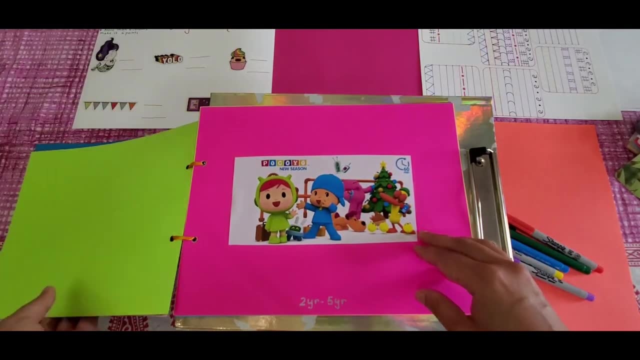 so i'm just giving you an example, because i have this whole book right here and let me just quickly flip the pages so that you know exactly what i'm talking about. and so he has all these cartoons that he's been watching for years. i have made a book for every year that he was watching.